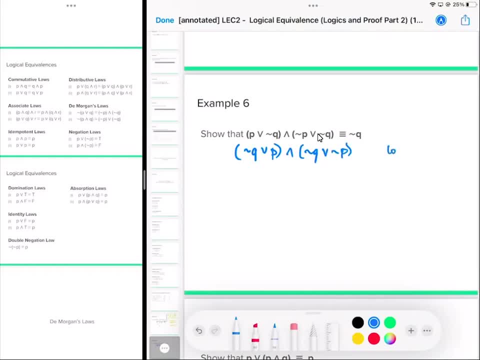 commutative laws, And now we can see that we can use a distributive law for this one. We have the not Q, not Q, and they are both being connected by the or in the operator. okay, So let us try. We have the not Q or P and not. 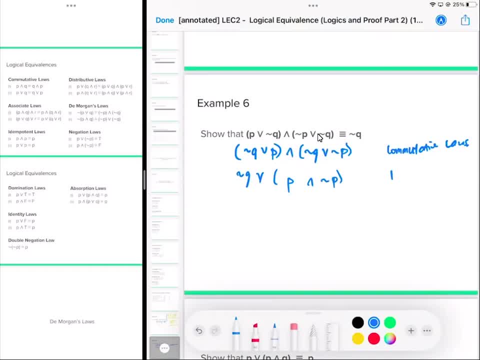 P. okay, We are using the distributive law. Again, you can do that because we have the not Q on both of the group statements and they are both being connected by the or in the operator. okay, Now the not Q, or and this can be evaluated into. 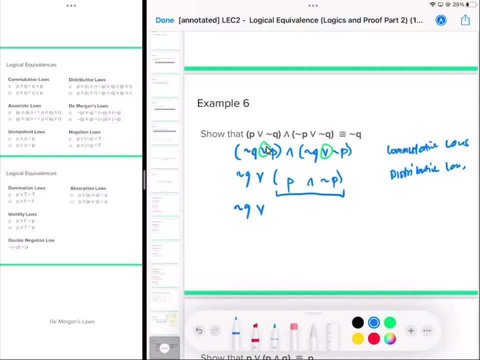 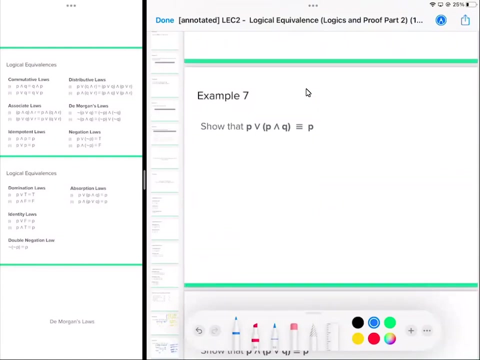 what This can be evaluated into: false by using the negation law. okay, So P and not P will result to false Now not Q, or false will result to not Q using the identity law. okay, Now let us move on to another example. We have P or P and Q is logically equivalent with P. 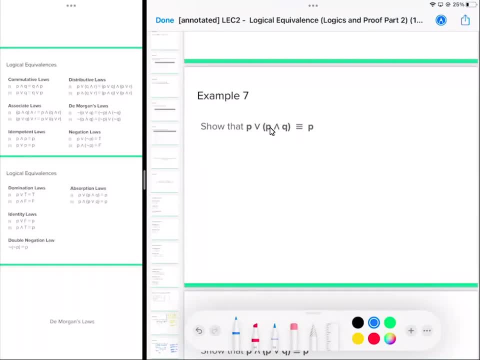 So is this familiar to you? So P or of group P and Q is actually the what. This is actually the absorption law. But we will prove this Using that this is indeed correct using the laws of logical equivalence. So at first look. 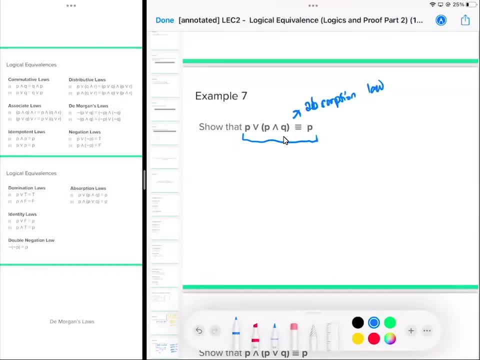 it is quite different to deduce how it was done right. But this P could actually be further used with other connectives. So we can use of the identity law. so we can use P and true for P and Q. Note that P and T will is logically equivalent to P or by.